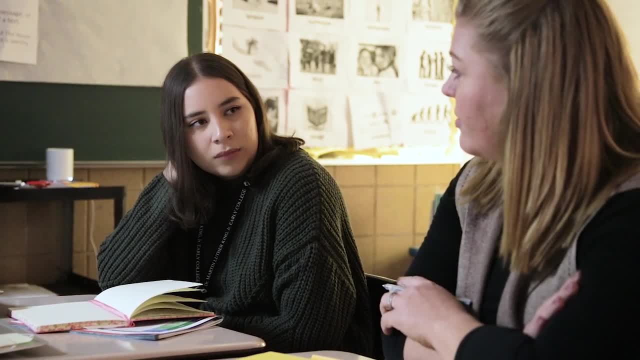 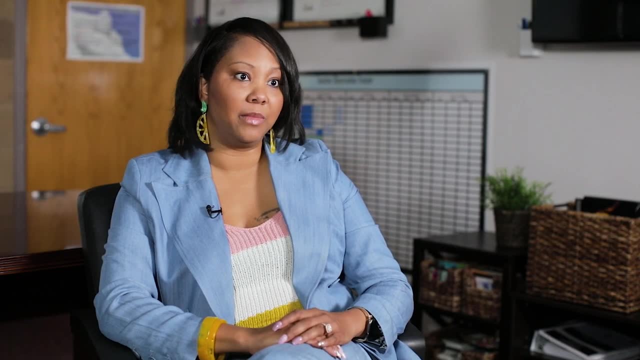 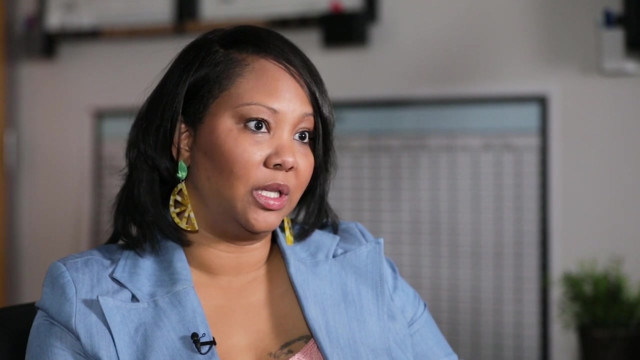 take a lesson that wasn't great and then help a teacher script a lesson that is. That's gonna be part of your action step today. Our feedback conversations last anywhere between 35 minutes and 45 minutes. They start with just providing that praise to the teacher. then we go directly into what we want: the 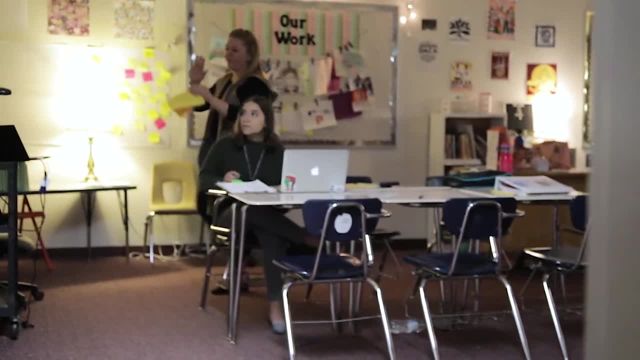 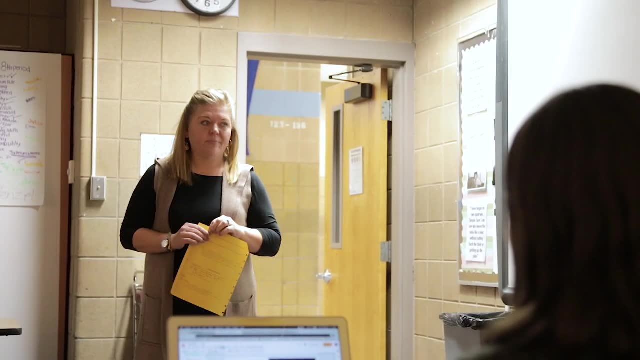 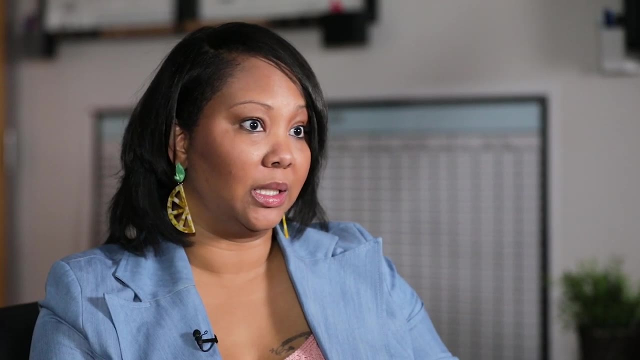 teacher to identify as their gap that was happening in the classroom. We provide the- whether that is the administrator or the senior team leap jumping up and being in full role-play, modeling or showing an exemplar teacher teaching, And we ask the teacher to identify the gap between the exemplar. 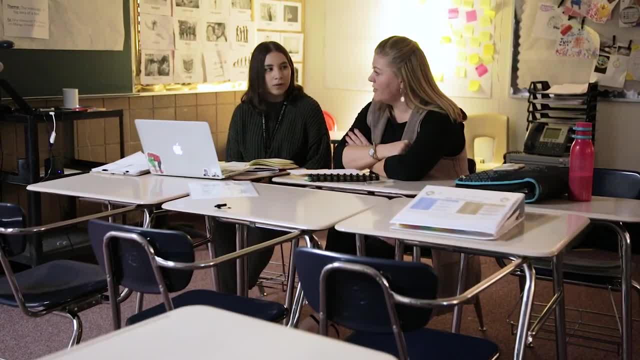 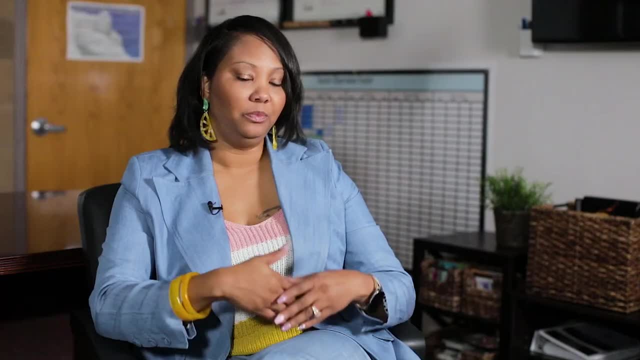 and what was actually occurring in their classroom, And then from there it kind of guides us into your action. step for this week is: and we identify the what and the how. Then we ask the teacher: where can we incorporate this in your lesson plan for next week? 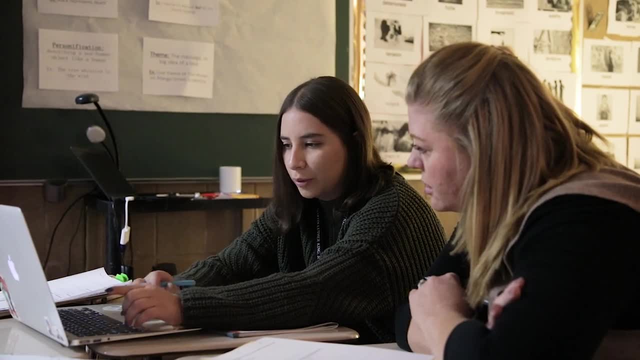 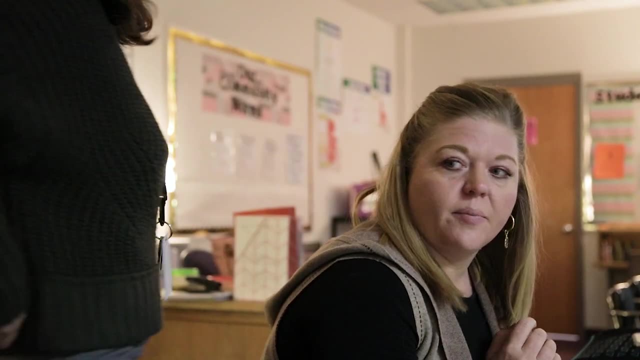 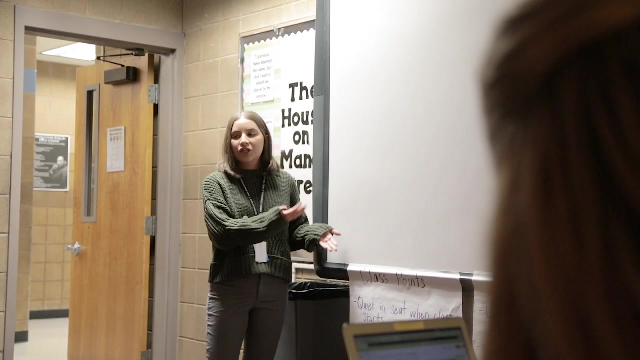 The teacher opens up their laptop, we identify the area and we give the teacher actually time during that feedback to adjust their lesson plan. Then we'll ask the teacher to jump up and get into full role-play and practice. Sometimes that's uncomfortable for teachers to be in a full role-play and practice. 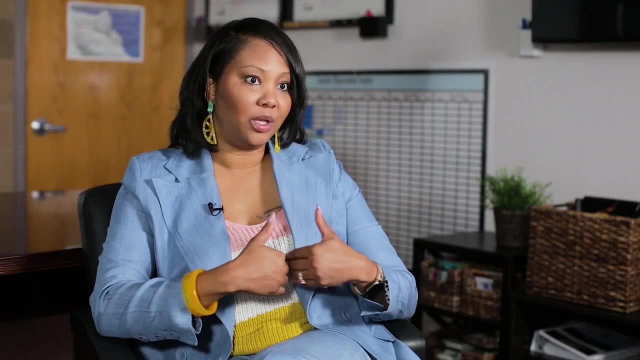 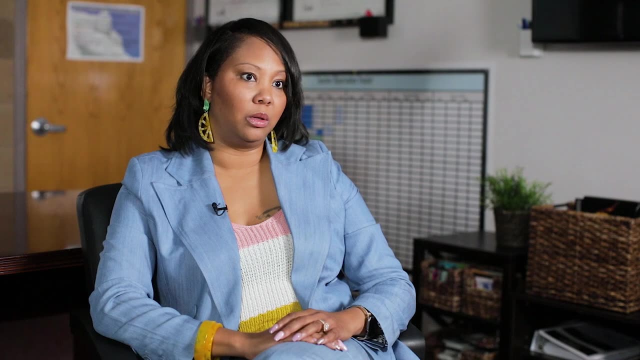 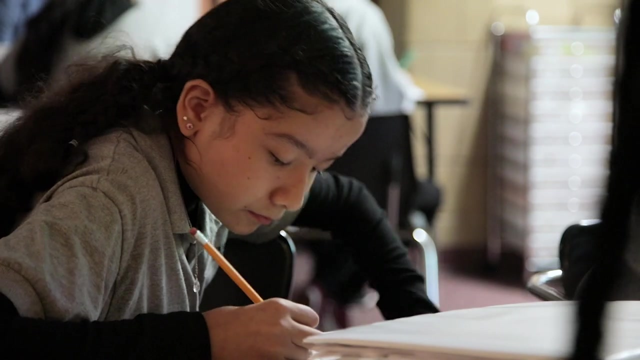 but teachers soon realize practice with us so that you can practice perfect with the students. I believe the observations and feedback has made impact with growing and developing And keeping and retaining our effective and distinguished teachers. So whenever you see a, I think I would be failing my students if I didn't have feedback sessions. honestly, 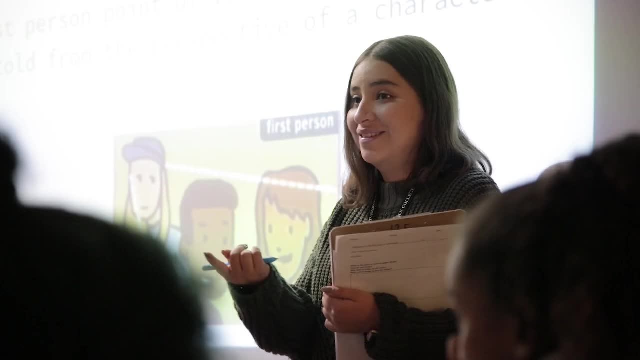 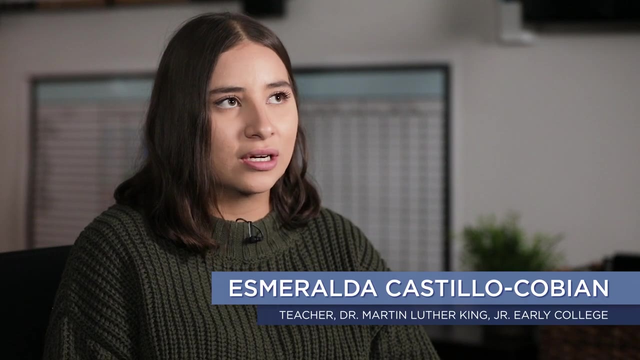 I had a lot of the elements as a first-year teacher that like I was supposed to have, but it wasn't necessarily as extensive as it needed to be before coaching. Like I remember my first coaching session I was like wow, like I'm doing all of this. 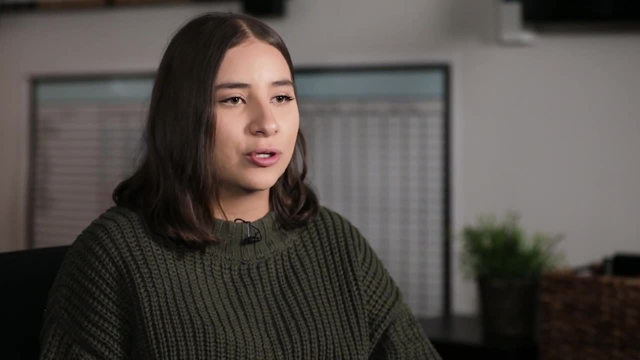 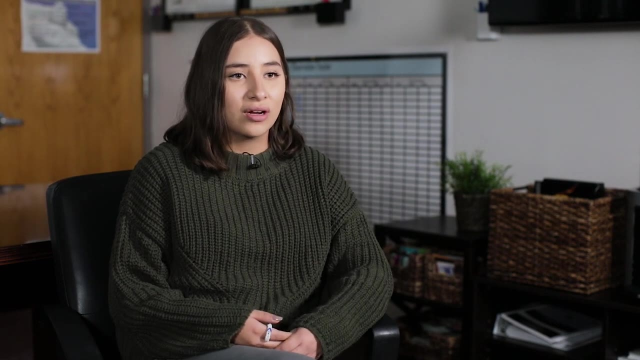 but I'm not doing it like to the extent, full extent that I could be doing to like support all of my students And now I feel like I'm more aware of a lot of things that I could be improving on because of coaching. All right, girl. 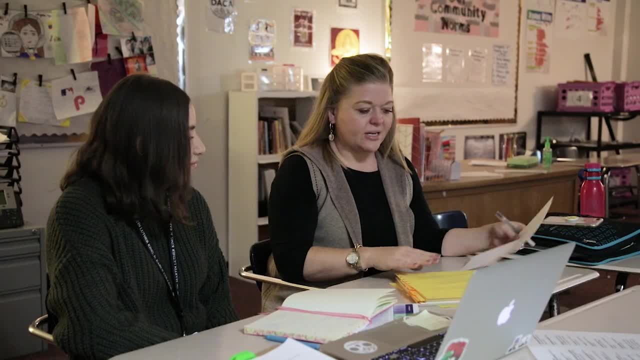 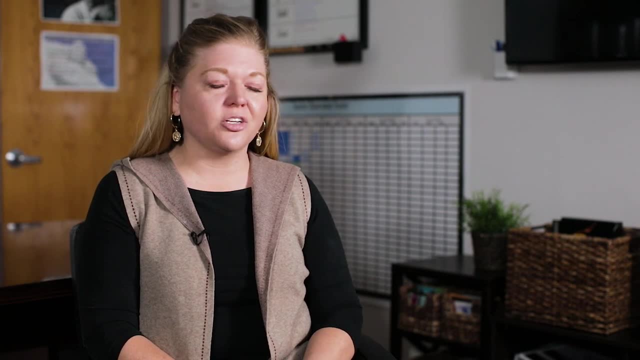 Sweet, Thank you, Thank you. Let me know how I go Shoot me a text When teachers email you or text you and they're like I did it. I feel much better about this lesson today, Like that small little change just made, like all the difference with the rest of my classes.